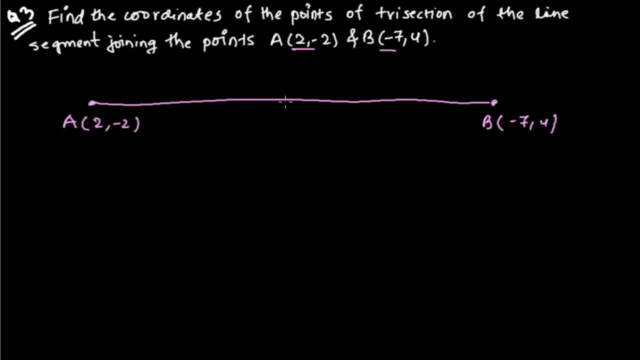 is negative, 7, comma 4.. So here are such two points. Suppose here 1 and here is 1, right. Suppose this is p and this is q point. This p and q point is dividing this whole line in equal three sections. It means question is saying trisection, right. So this is equals to. 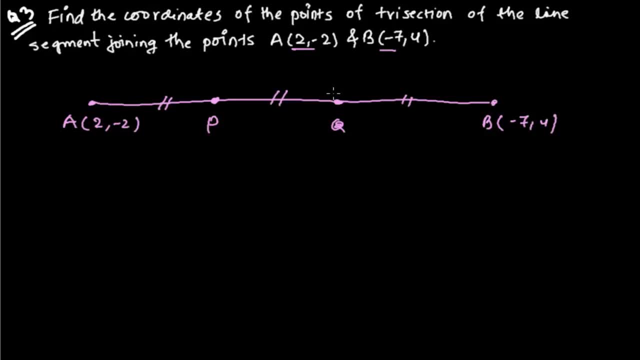 this is equals to this. I mean a, p is equals to p, q is equals to q, b right? So we need to find out the coordinates of this p point and q point. Let me say this point is x 1, y 1 and this: 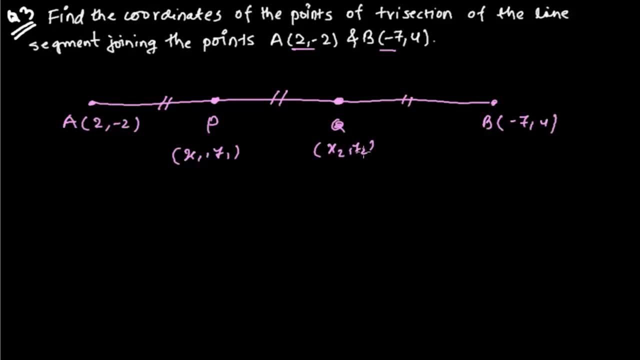 q point is x 2 and y 2, right? So I need to find out the coordinates this p and q. So if I want to use the section formula, then I must know the ratio by which it is cutting this right. So 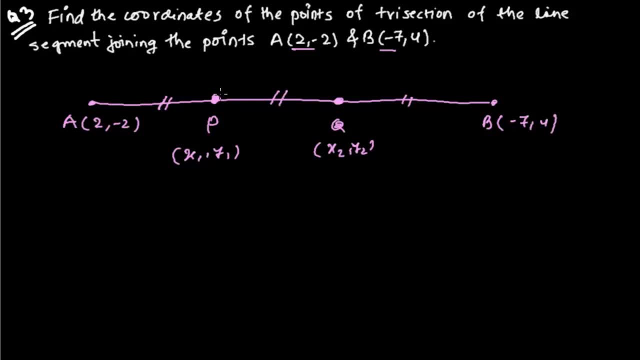 this part, this part, this part, there are three equal parts and we can say: since this is two equal parts and this is one equal part, So this is one part and this is one and two equal parts. That's why it's two equal part. So what can I say now that this p point is dividing this a b line in? 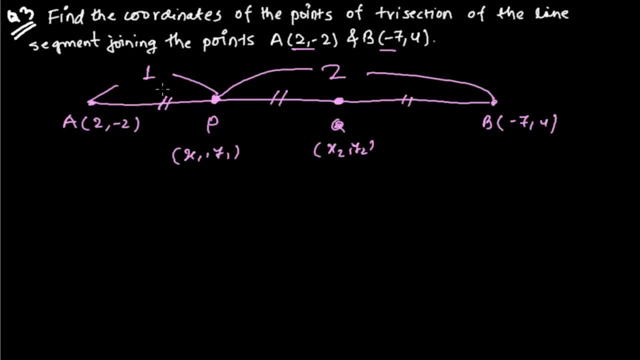 the ratio of one ratio two right. One ratio two. this p point is dividing. And if you talk about this q points, then see, in left side there are two equal parts, right. So if you come here, right, If you come here, there is two equal parts, I mean, yeah, And here. 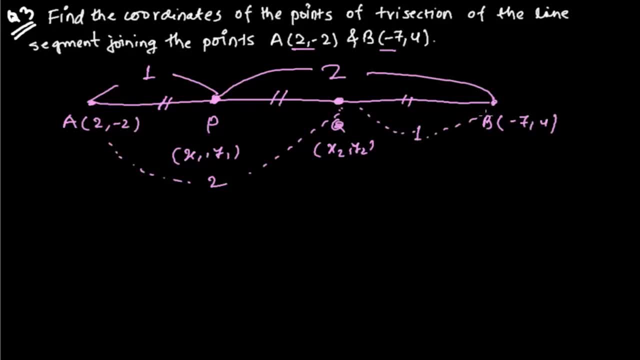 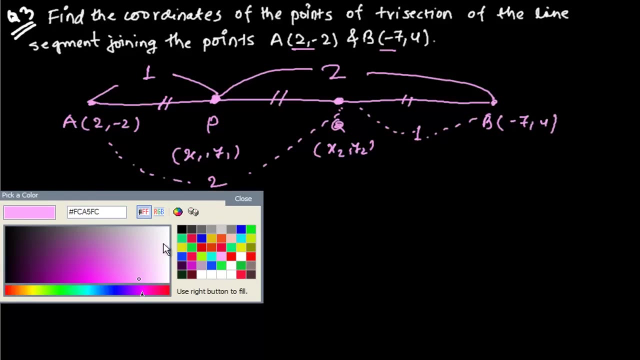 is one equal part, right? So this q point is dividing this a- b line in two, ratio one. and this p point is dividing this whole a b line in one ratio two, right? So let me first find out the value of this, this, this p point, I mean the coordinates of this p point, right? So let me? 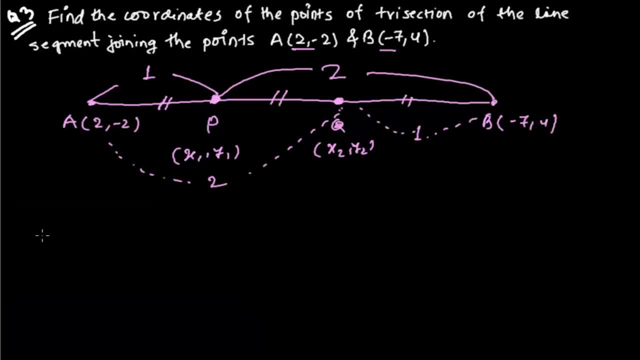 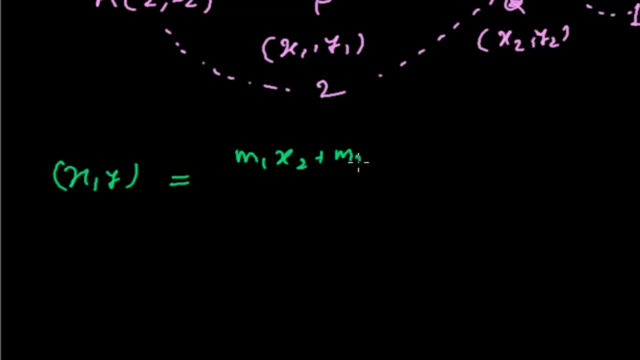 find out first. okay, So let me write first the section formula, that is x comma y is equals to m 1 x 2 plus m 2 x 1, whole divided by m 1 plus m 2.. Again, m 1 y 2 plus m 2 y 1. 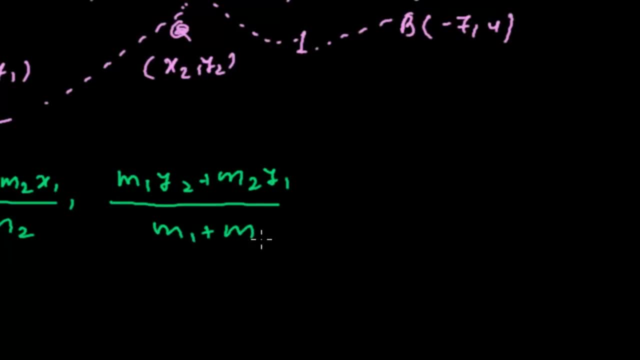 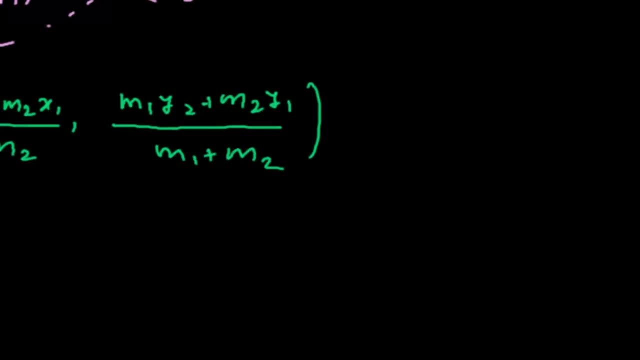 whole divided by m 1 plus m 2, right, This is our section formula. Now I'm applying this section formula in this, in this problem, right? So let me first find out the p, that is x 1,. 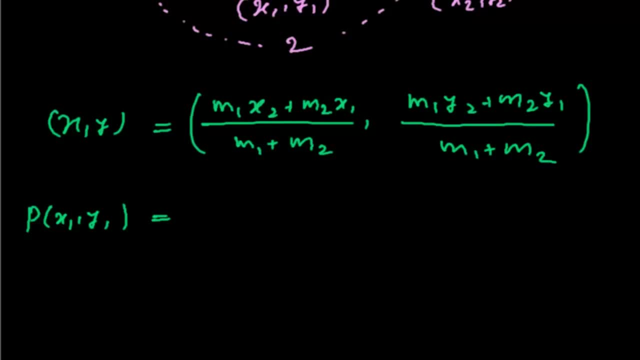 y 1 is equals to m 1, x 2.. So let me suppose this is this point- is x 2, y 2 and means here for this formula only x 2, y 2, and this will work as x 1, y 1.. So m 1, m 1 is here 1.. So 1 times. 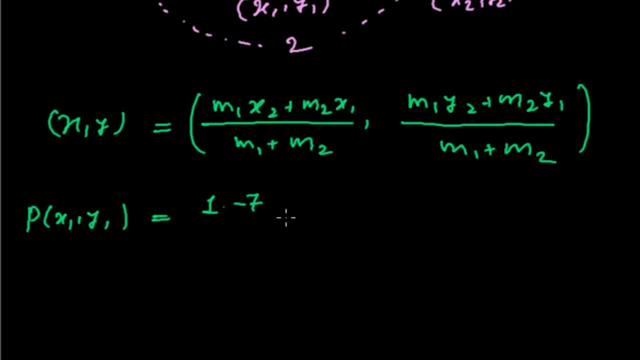 x 2,, that is minus 7, minus 7 plus m 2.. m 2 is here 2 times x 1,, that is 2, right Whole divided by m 1 plus m 2, that is x 1, y 1.. So let me first find out the p point, that is x 1, y 1.. So 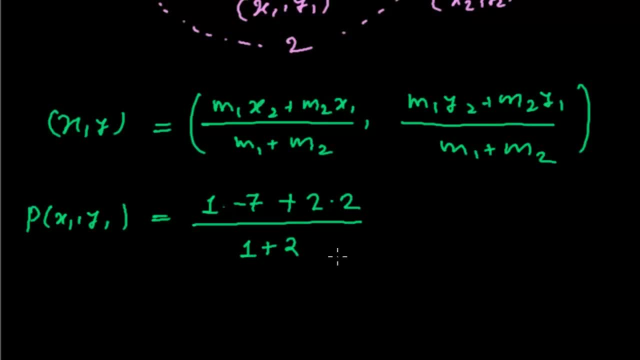 m 1 is 1 and m 2 is 2 plus 2, right, And again m 1 y 2.. So m 1 is here 1 and y 2. here is 4 plus m 2. again here, 2 times y 1.. y 1 is here minus 2, that is negative 2, right Whole divided by m 1. 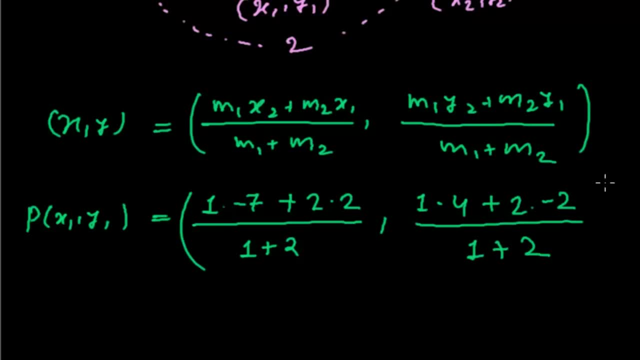 plus m 2, that is 1 plus 2 again. right? So again, p x y is equals to 1 plus m 2, right? So 1 times minus 7, it will be minus 7 plus 2 times 2,, that is 4, whole divided by 3, right Again? 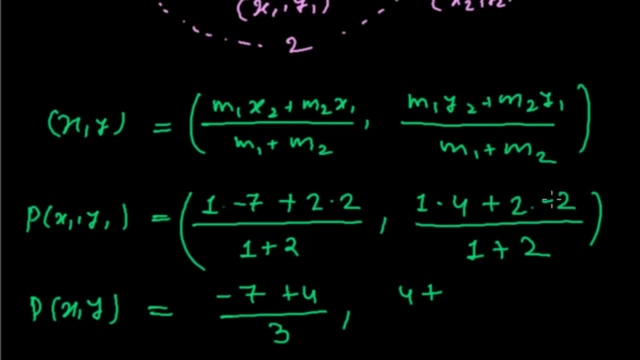 4 times 1,, that is 4 and 2 times 2, but negative, So it will be negative. 4, right, So negative. 4, 1 upon 2, right. 1 plus 2,, that will be 3, right. So what we got here, that. 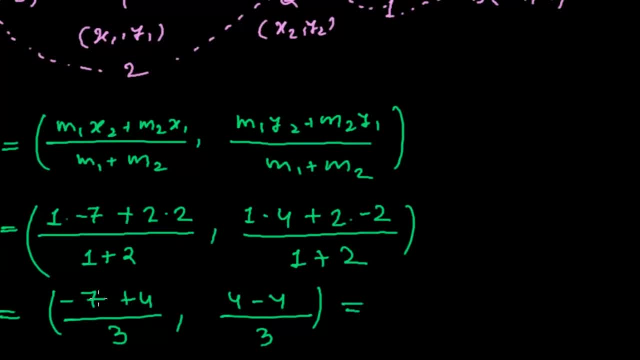 minus 4 plus 4.. So plus minus, it will be minus, always the sign of the greater, and the operation will be negative. Also, it means a minus will be, So 7 plus 4 will be 3 here. since it is negative, So negative 3. 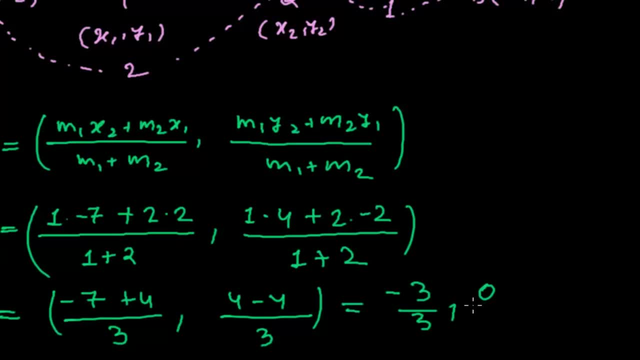 divided by 3 and 4 minus 4, that is, 0 divided by 3, right, So it will be minus 1 comma 0, right, So we got the value of this point. that is, negative 1 comma 0, right. Now we need to. 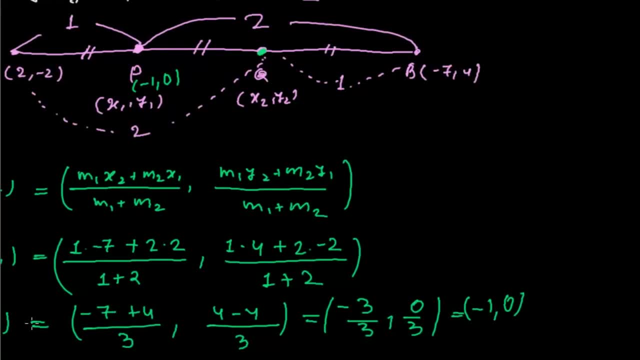 find out the value of this point. What is the value of this point? q right, Fine, this color is the best right. So see here, friend, if you want to do with the section formula, that is, 2 ratio, 1 also. 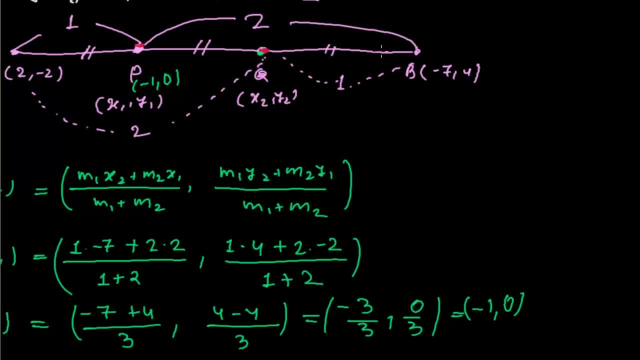 it is also right. And if you want to do this here, see here: p and q, right, So here pq is equals to qb. So I can say that the point q is the midpoint of this pq line, right, Sorry, pq line Only see. 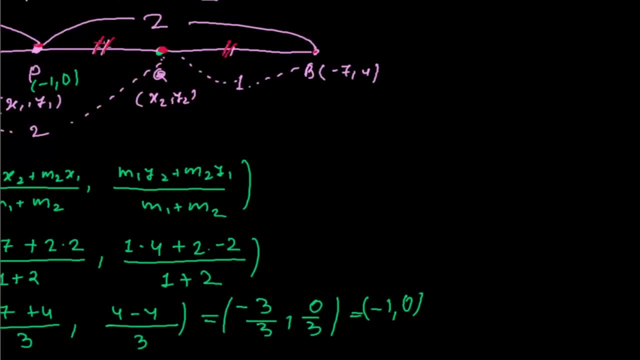 this much right. Only see this much here. This q point is the midpoint of the pb line also, because this part is equals to this part. So I can use the section formula, as I used to do, or I really do here, I just do like this, or I can use also here the midpoint formula, right? So I think 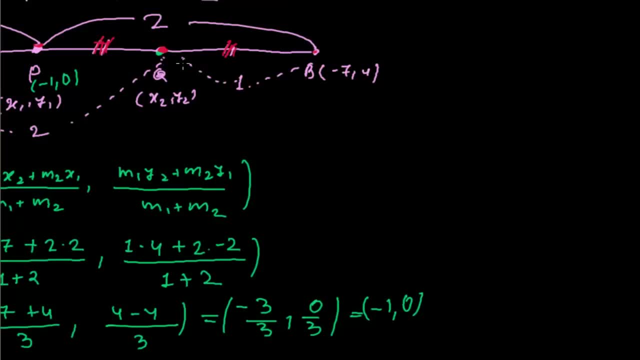 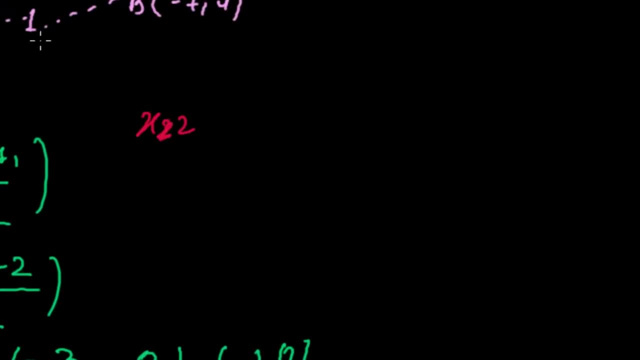 midpoint formula is the best for here, right? Midpoint formula is just the average of these two points, right, The middle point, right? So let me use here midpoint formula. that is x2,, it is x2, let me write properly, okay, The q point, that is x2 comma, y2 is equals to right Midpoint formula. 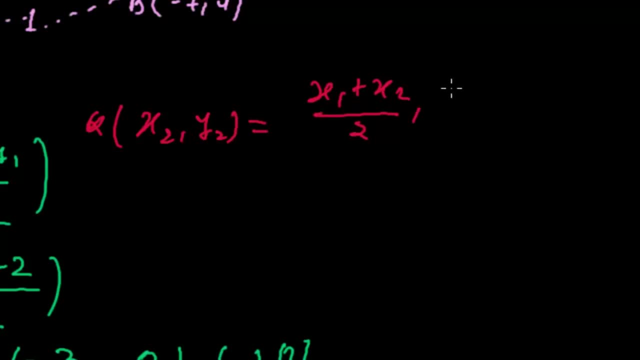 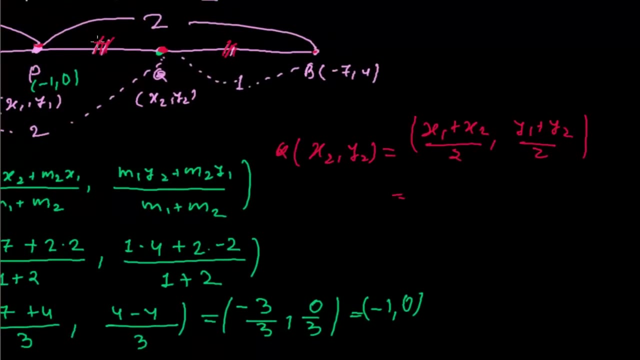 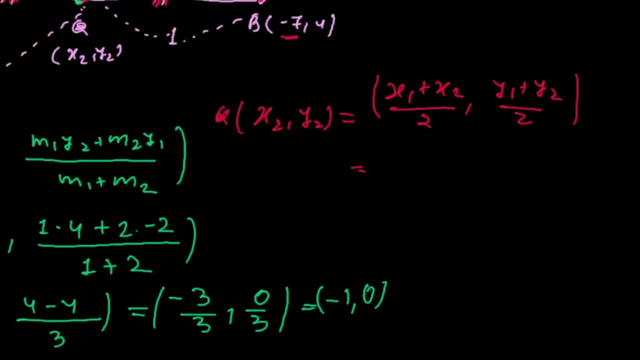 I am applying here x1 plus x2 upon 2.. Again, y1 plus y2 upon 2, right. Or we can say that just average of these p points. So average of x coordinate, that is minus 1 plus right, Minus 1, and this minus 7.. Average of this x coordinate. 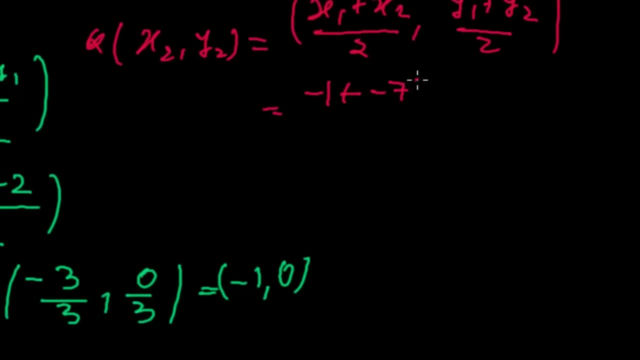 that is negative 1 plus minus negative 7, all divided by 2, and again y1 plus y2, or the average of this 0 and 4, that is 0 plus 4 divided by 2, right, So it will be minus 1,. 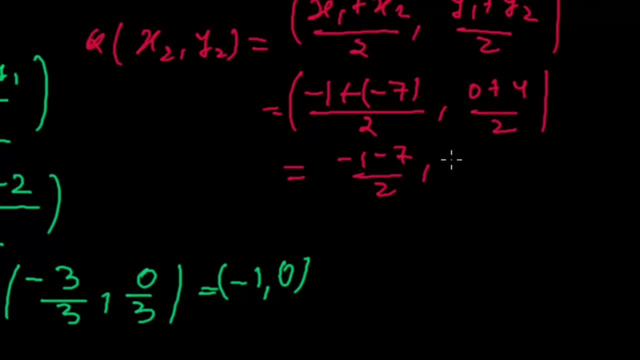 plus minus minus 7 upon 2, 4 upon 2, right. So it will be minus 8 upon 2, again 4 upon 2, that is 2, right. So overall what we got, that the q point is equals to minus 4 comma 2, right. 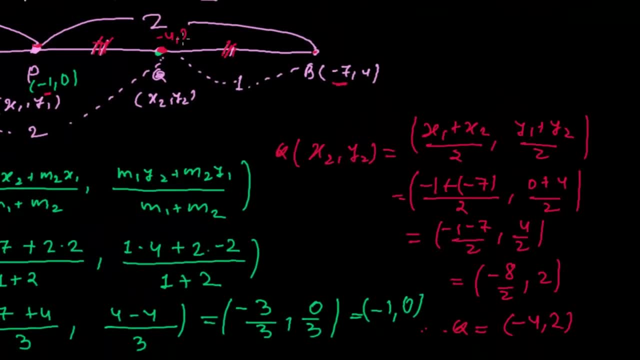 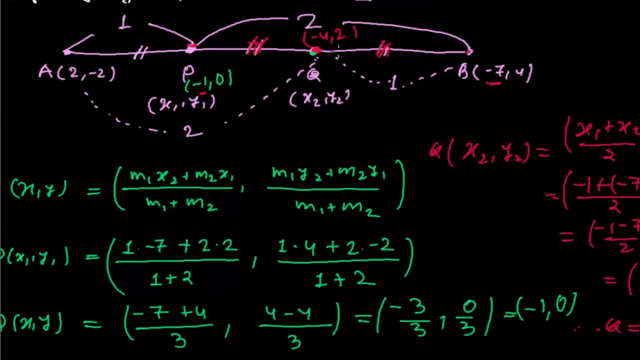 So we got the value here, that is minus 4 comma 2.. So we got the answer here that here the line was a, b and the two points here, p and q, was trisecting this line. so p point we got that is. 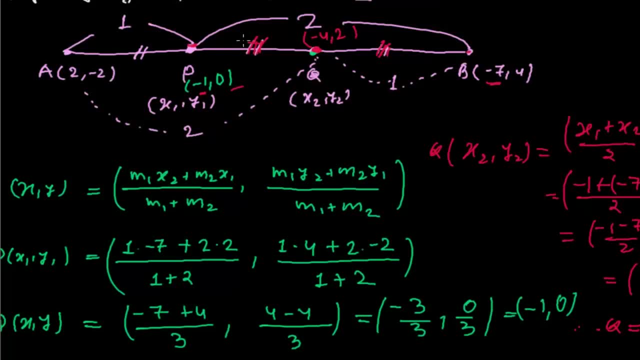 minus one zero, and the q point is minus four comma two. so like this we have to solve this kinds of problem. all right, either the line is uh, dividing into four equal parts, or five equal parts, or seven equal parts. we just have to first find out the ratio, in which ratio the points are being cut.